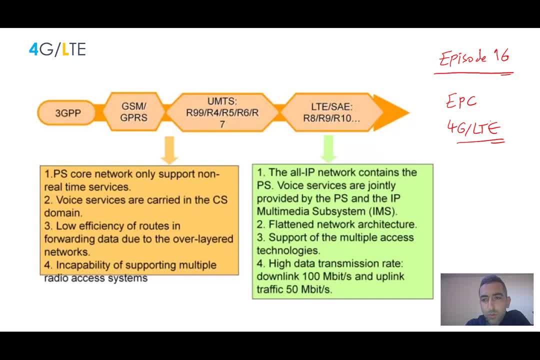 we should discuss that. what was the motivation for the, for the immersion of this generation of mobile networks, LTE, which is long-term evolution? As you know, LTE is 3.9G but commercially, according to the acceptance of 3GVP, we accept that we can commercially say 4G LTE. As you know, many of these 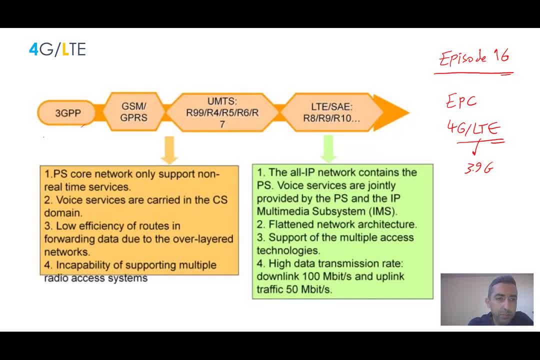 standards are generated by successful 3GVP third generation partnership project And until release 7 we had GSM, that was 2G, GPRS, the packet switch of the packet switch of this generation. After that UMTS for 3G we have some. 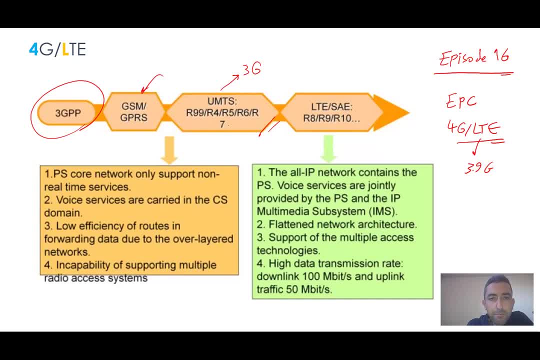 release R99 to R7.. For example, in R4 we had the separation of CP control plane and UP User plane, for example. I think that I have discussed this in the previous episodes about separating MSC from media gateway. As you know, MSC is responsible for control plane and media. 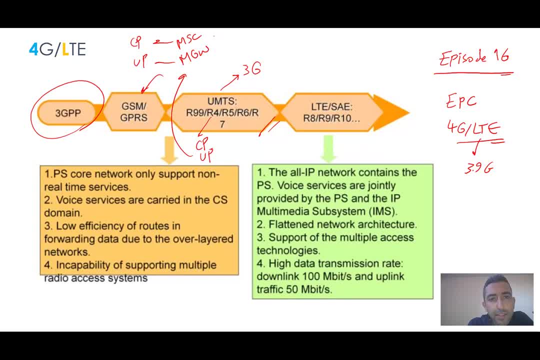 gateway is responsible for user plane And in this And in this network structure here usually use H2O-Done Ports, H248 protocol or mega and in release 5. the important thing that happened in release 5 was introducing IMS, IP multimedia subsystem and so on. which IMS? 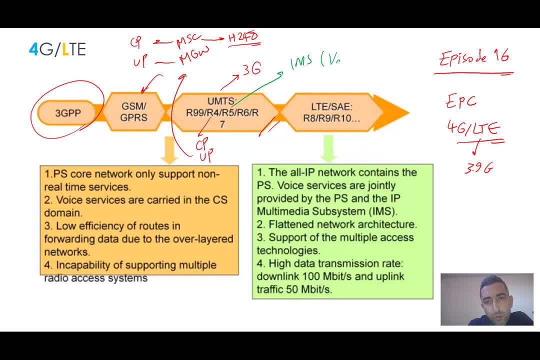 was is responsible for handling voice over LTE service and in the later episodes I will fully discuss about this. IMS and Volta service. okay, for a brief discussion about the release. and if maybe some of you don't know about this, we have beside generations of the mobile networks which all of you know that from. 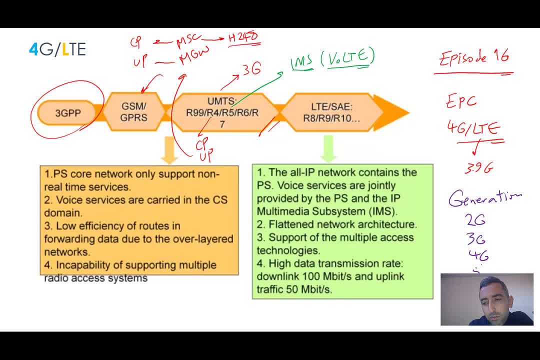 2g, 3g, 4g, 5g and now and now, the study of 6g. we have also some release that started with our 99- oh sorry, I started with our 99- and right now our 4. right now, I think. 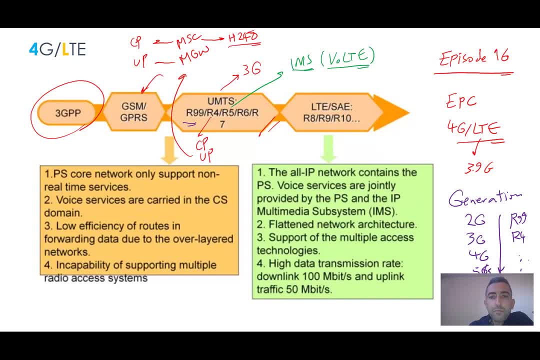 we are on our 17. okay, but from here, from 4LTE, long term evolution and system architecture evolution. we have these releases are eight of nine, r10 and so on. so let's have a look at the motivations of uh emer, immersion and generation of these mobile networks in 4g- okay, we see in in the previous generation, in 2g, 3g. 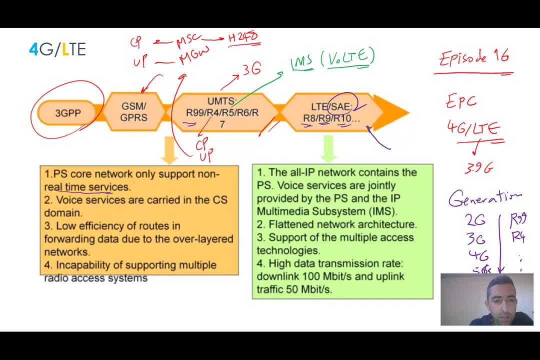 ps core network only support non-real-time services, but in 4g lt we have the all ip network and many real-time services. we have the all ip network. it is very important the all ip network contains the ps and voices are jointly provided by the ps and the ip multimedia subsystem. 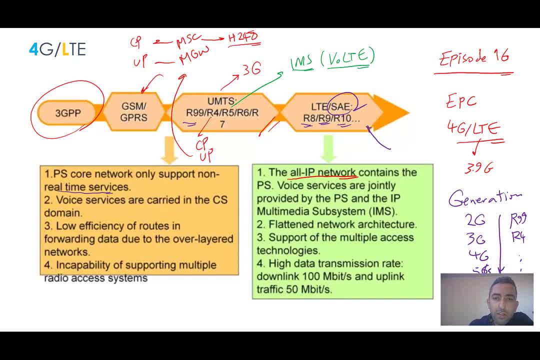 as i told to you um before we have a in release five and during the three g time ims was introduced but infrastructure and the speed and the network infrastructure was not enough and was not mature for this service. but we see that in when we had lt, the volta service and ims was commercially usable. another thing that we can say that 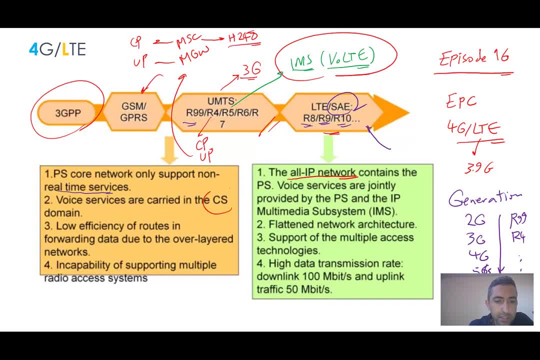 in the previous generation voice services are carried in the cs domain, but now you can see that voice can be handled in ps and in the volta. all of the packets are sending via the, via the packet core network and ims and the signaling goes on the ims core network and also we see that these 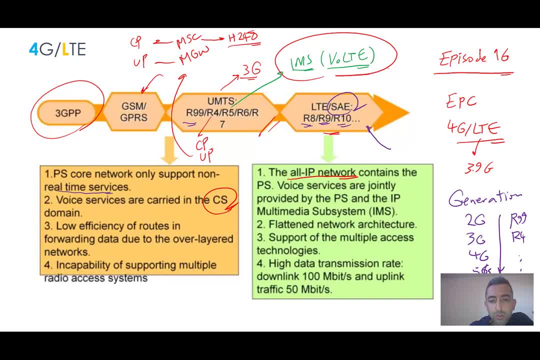 new networks. epc evolve packet core in fourth generation. it's simpler and flattened network architecture, support of multiple access technologies and theoretically the data transmission rate is about 100 megabits per second for downlink and about 50 megabits per second for opling. but, as you know, in some countries, maybe in these these- 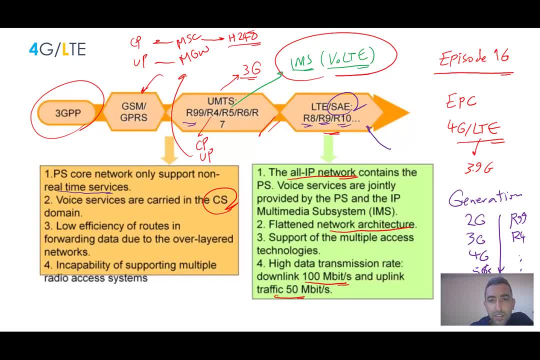 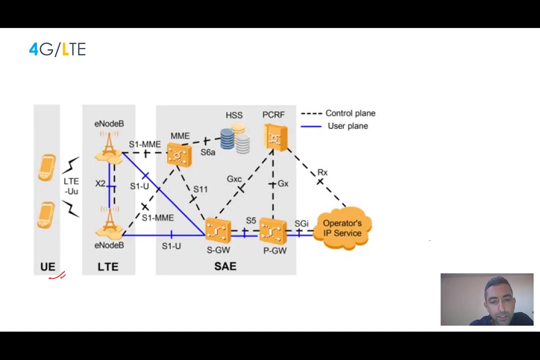 maybe very fewer than these amounts, but this is ideal, ideal, okay, this is a some brief comparison between the previous generations before for glt and this generation. okay, you can see in this picture we have separated the network to three different part. here is UE or user equipment. in the previous generations we 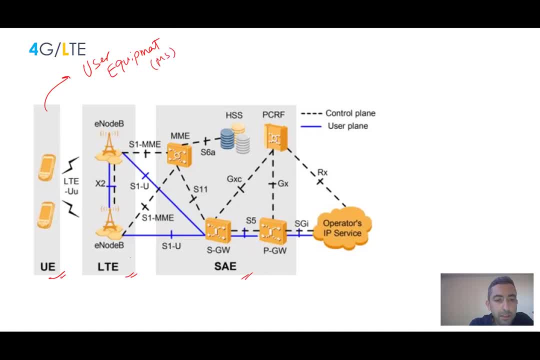 told mobile subscribers to this also. here we have long term evolution, which is which described the radio part. you see that before, in 2g we had BTS for the last access space station based transceiver station and we had BSC for controlling this BTS. in 3g we had not' be and RNC. 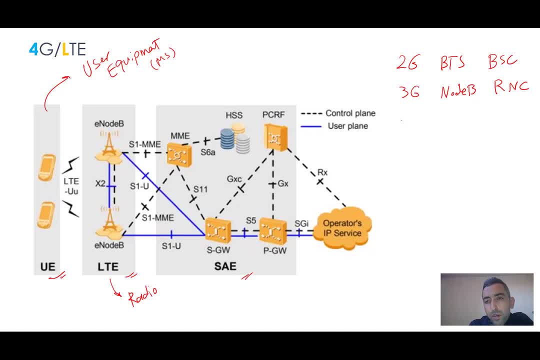 radio net for control like this. but in 4g lte, both of them evolve and one node we have that is e, not b. also in 5g we have g node, okay i, i don't know what would be the name of the 6g, maybe in the. 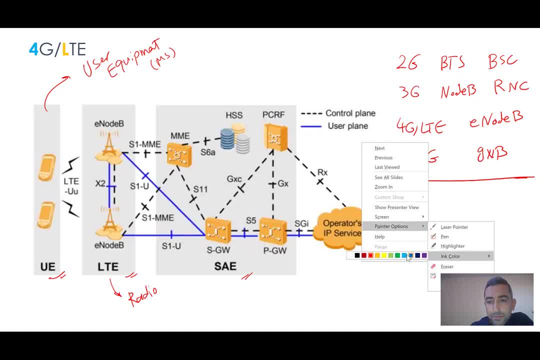 future. i introduced to you- uh, okay, so, and you see that we have, you know, be here- and many other network elements that i will introduce to you. but in this episode we just want to have a big picture and introduction to you. maybe this epc lessons continue for three or four. 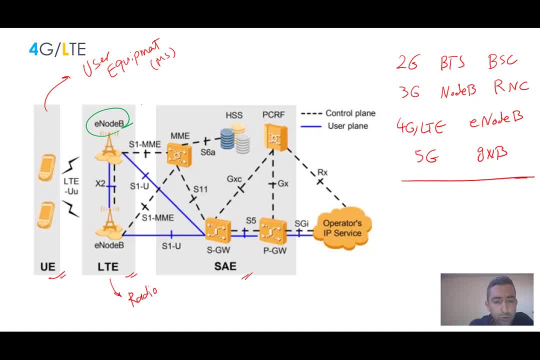 more sessions. as i told you before, we have also some interfaces between every node in the network. you can see, for example, between e- not b and mme, the interface is s1, mme or s1c, and here, between e, not b and s gateway or sgw, the interface is s1u. but i told you also before that. 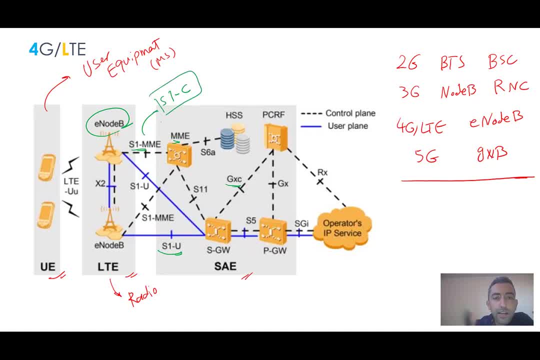 beside this interface, we have also a protocol and protocol stack which you, which you should care, take care of them. for example, in this, in this example, s1mm or response c, the protocol is what protocol is spawn, ap. and you should also know the protocol stack which i draw for you here. 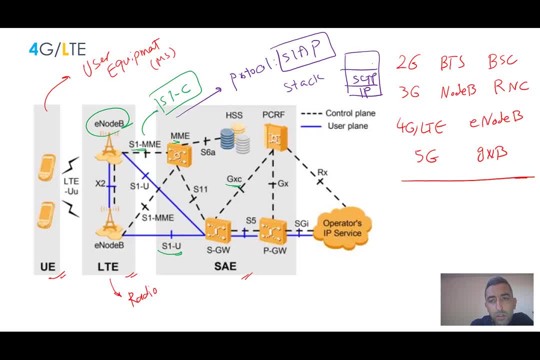 ip, sctp, s1ap, and a sub layer will also be here which the name is nas- non-access stratum. that i will discuss it later. and we also have some something about user plane. as you see, user plane and control plane. these these lines are responsible for control plane and the blue line is for user plane. 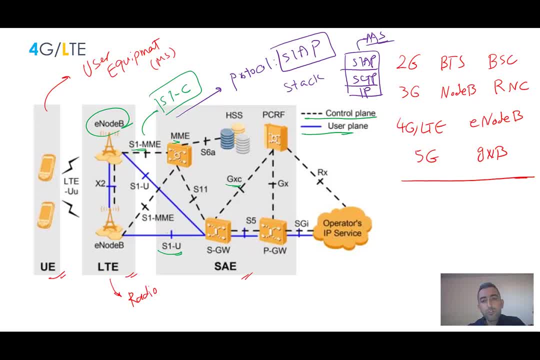 from now on you should take care of control plane and user plane. control plane is responsible for signaling and user plane for the service. okay, let me change the color of my marker. okay, so we have got the cell so that we take it and move it here and now we're going to use the gearsharing solution to see what work. 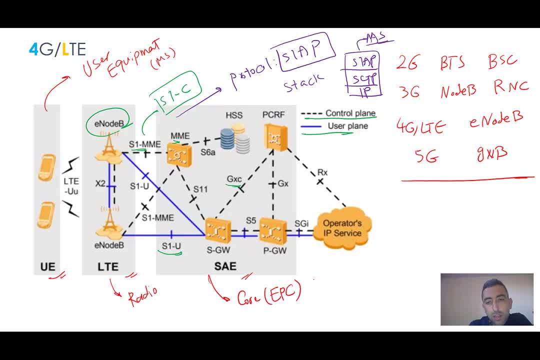 and scan, thats get all the user. finally, they areア⟭⟩. and we also have gearsharing. doin i here stop again. and this will work in cascades. also, and this is also a default system, sepsis. uh, we need to use, uh, the four glt networks. so here also the radioport, and here is the core part of 4yltnetwork which we can tell it epece and here is the core part of our network which will tell it epece: evolve, evolved packet core. and all of this system is named\'85,, 1900,00,00,�� was called daficiente- eps- evolved packet States. and sec Masking system, EPS- evolved package system. this is the cost of the system called Patura, with this leadingW bags. our same system is the temples: eps, evolv packet system. 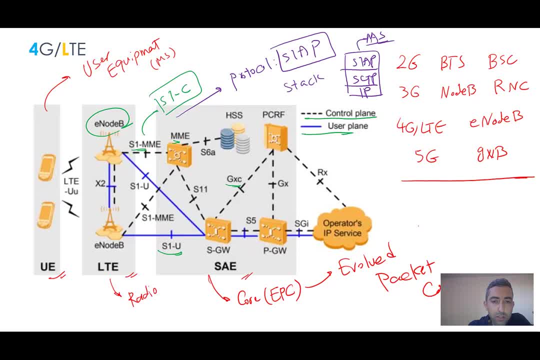 Also, you can see that EPC Evolved Packet Core contains of MME Mobility Management Entity, SGateway or SGW, PGateway or Packet Gateway, PGW, PCRF Policy and Charging Rule Function and some other networks that we can see here, for example, Operators, IP Service. 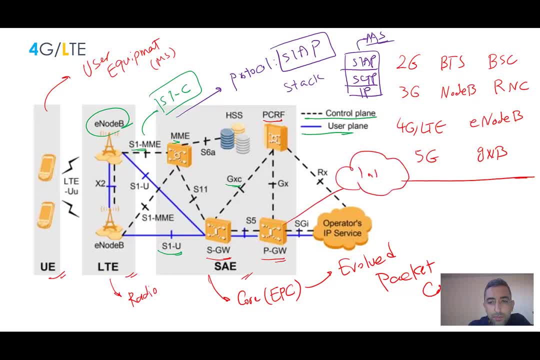 or Public Data Network, maybe Internet or maybe IMS Network, which is responsible for the Vault service. Okay, because from now on I want to make some more short videos, but several more Short videos, but several more videos. I think for this session is enough. 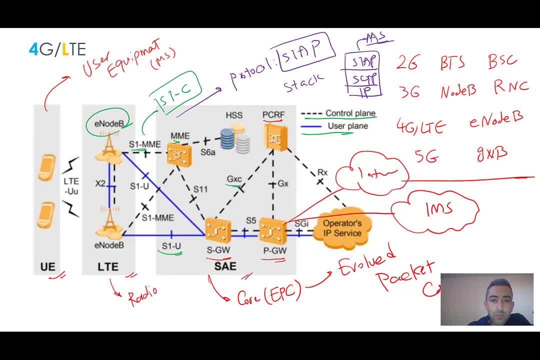 But in the next session I will go through the details of each and the function of each network element and we will discuss it in detail. I hope this video would be informative and useful for you and hope to see you in the next videos. Bye. 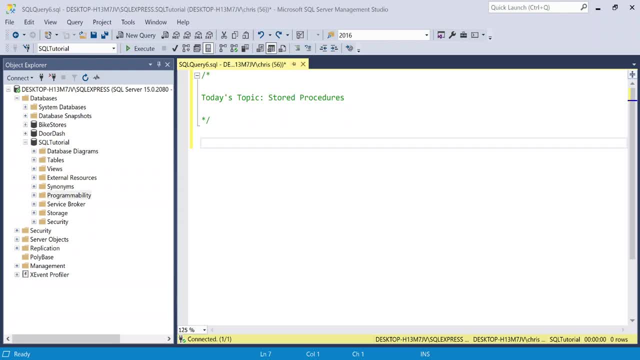 What's going on everybody? Welcome back to another SQL tutorial. Today we are talking about stored procedures. Now, what is a stored procedure? A stored procedure is a group of SQL statements that has been created and then stored in that database. A stored procedure can accept: